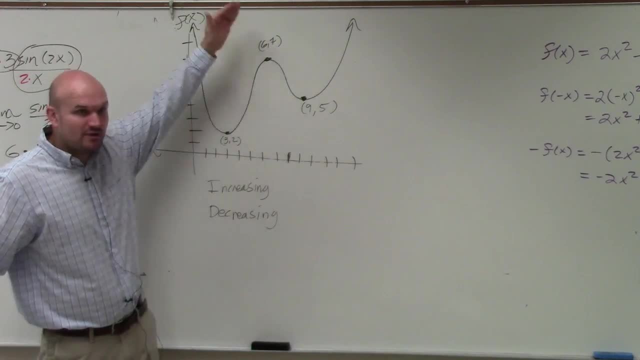 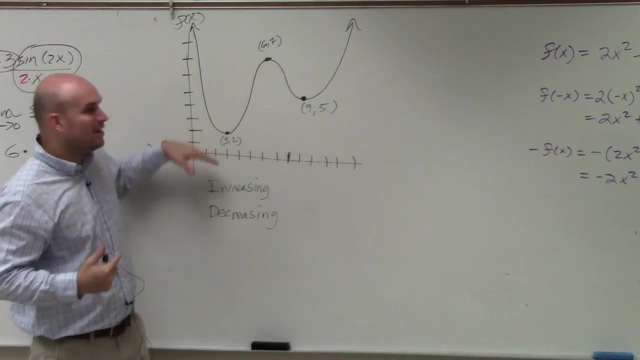 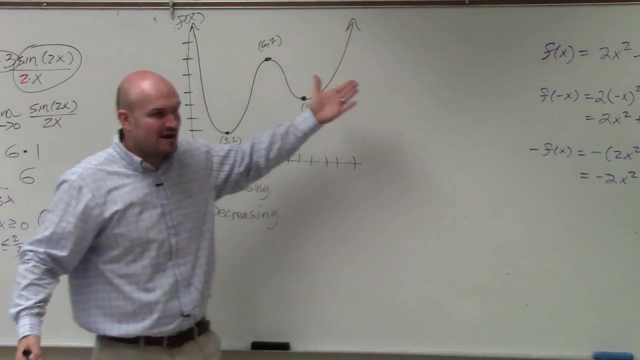 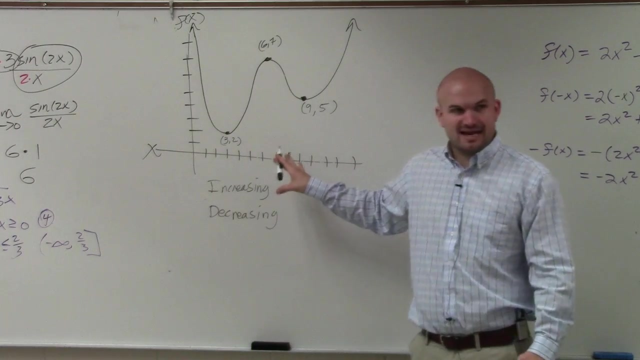 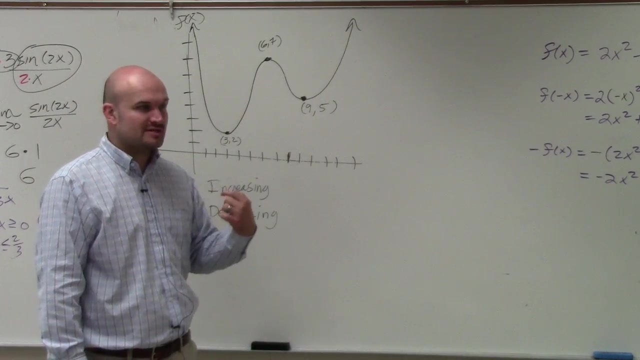 F of x values. That's telling us where the graph is going up or down: right X goes, left or right. We're going to read from left to right. We want to be careful, We want to watch what is f of x doing. When f of x is going up, f of x increases. As f of x is going up, the graph is increasing. As f of x is going down, the graph is decreasing, right? We see that f of x is not remaining constant anywhere. All right, So now that we know when f of x is increasing, we're looking at when f of x is increasing or decreasing. So let's start from the 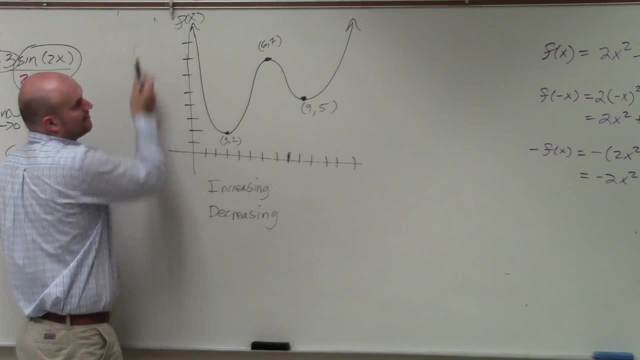 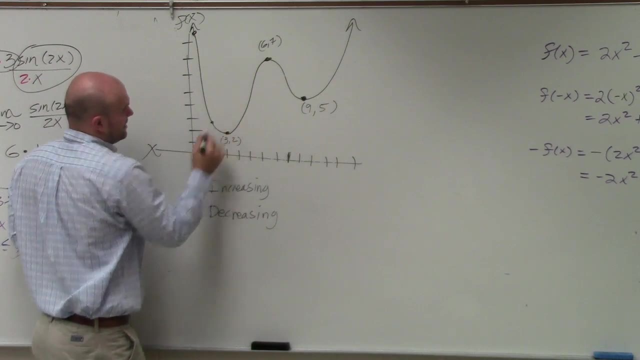 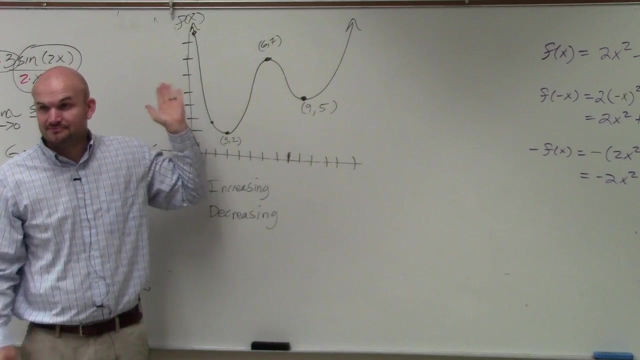 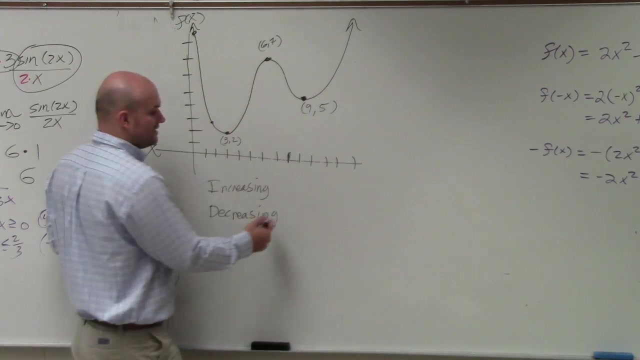 furthest left. We know this graph is going to go up to left. So as we start here, as we start moving to the right, we kind of maybe pick, like some points, Point here, point here. So, reading these graphs from point one to point two, what is the behavior of this graph? Is it increasing or decreasing, Decreasing? It's pretty obvious, right? You can see that the graph is going down. Here's how we're going to write that. We're writing the graph as its x values. So from the x values it's decreasing. 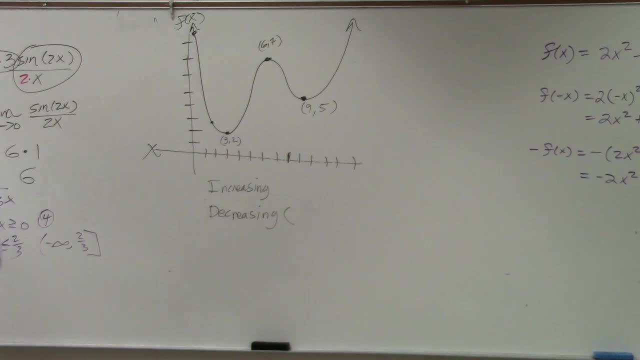 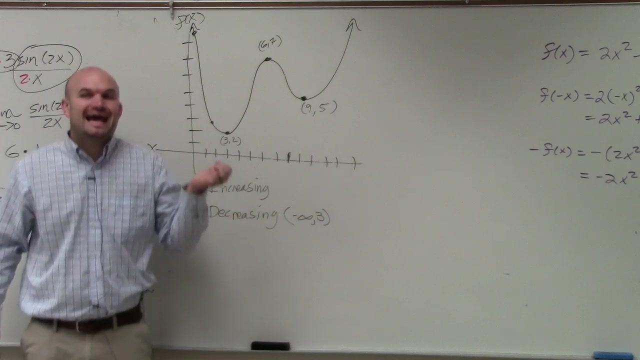 Sorry, From the x values f of x decreases. So what are the x values that it's decreasing? Well, we don't know how far on its left it's going to go, So we're going to say negative infinity. So how far does it go until it stops decreasing? How far over does it go? Three, OK, Then. from the x value three to the x value six. 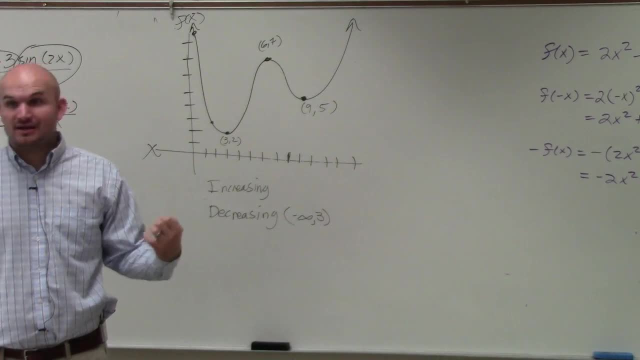 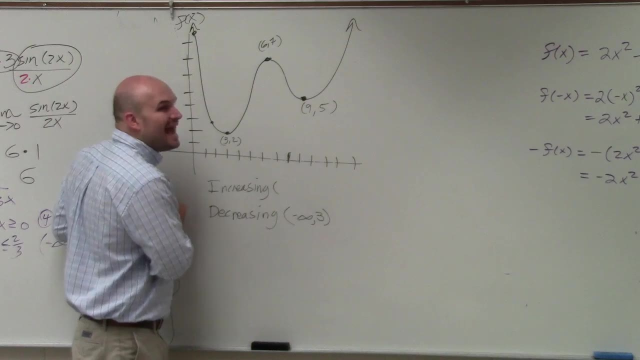 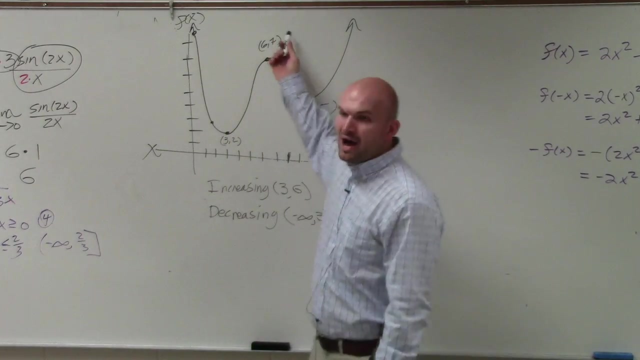 is the graph increasing? Is the f of x increasing or decreasing, or constant Increasing? So what we would write is: the graph is increasing from the x value three to six. The most common mistake is everybody wants to put in the y values. The y values is what we're just watching. We're just 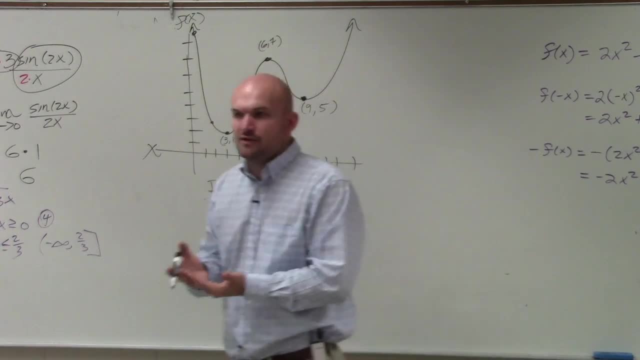 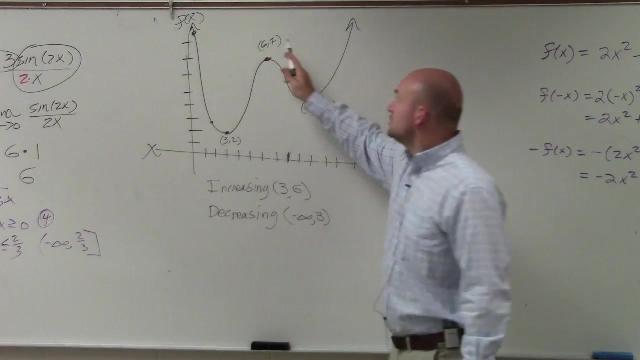 watching if the y values are going up or down. But we're writing the intervals of the x values because we're concerned about we're decreasing interval of when x of x increases, f of x either increases or decreases, So then we continue. So from the x value 6 to the x value 9,.